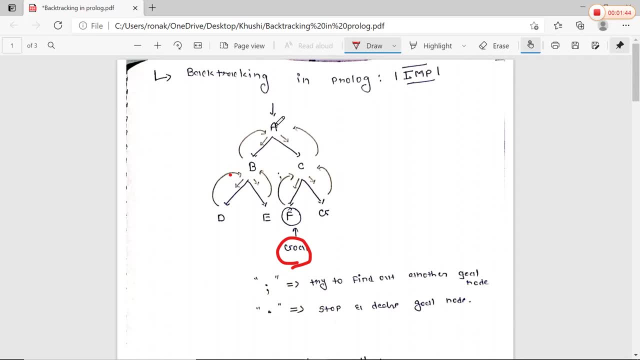 From the A node we have two options. First we move a left, After that we move a right. So here we move a left. First of all we move left, So here we move A to B. After that, when we reach B point, then we have again two options: D and E. 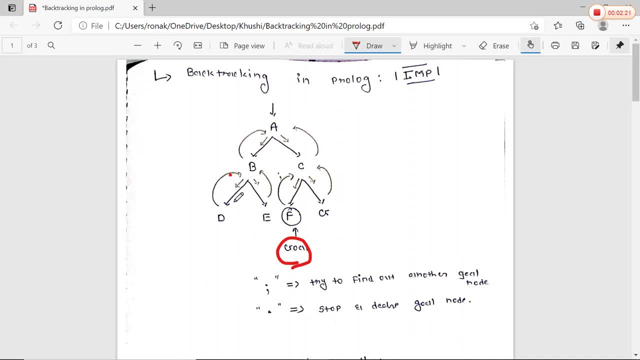 So first we move to the left Means, we move to the left side of B And we check: D is our goal node or not? If yes, then quite Otherwise we have to backtrack. So here we go: A to B, B to D, From D to D. we came to know that this is not our goal node. 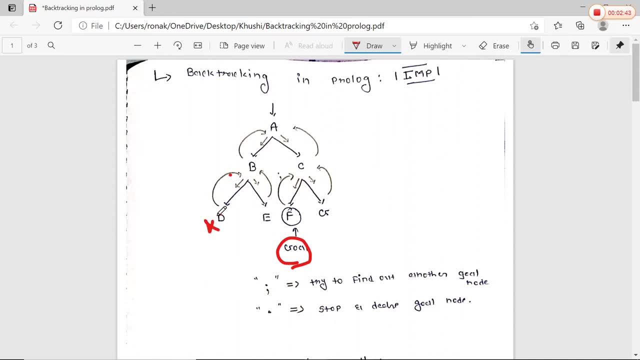 Okay, this is not our goal node. So what we did? We backtracked it. After backtracking, what did we get back? We came to B Again. we have one option from B- That was the right side Means B to E. So we checked E. E is our goal node or not? So what did we do? We went back. 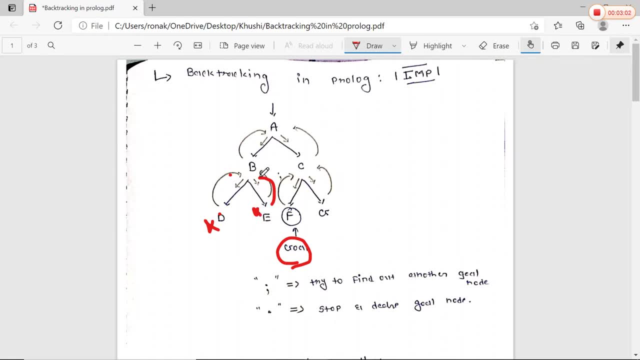 That means we also cancelled this node. Now what do we have to do? Now? we have to check that there is a third option, of B2, but there is none. So what will we do? We will backtrack from there Means we will move B to A. 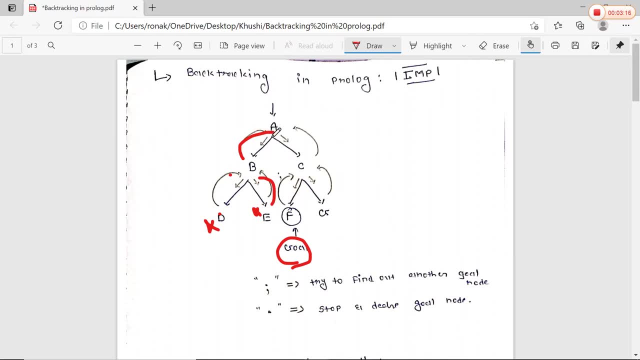 Now, what do we have to do? The other side of A means, right hand side. we have visited this node. Now what do we have to do? Right hand side? Now we have to check that there is another node. 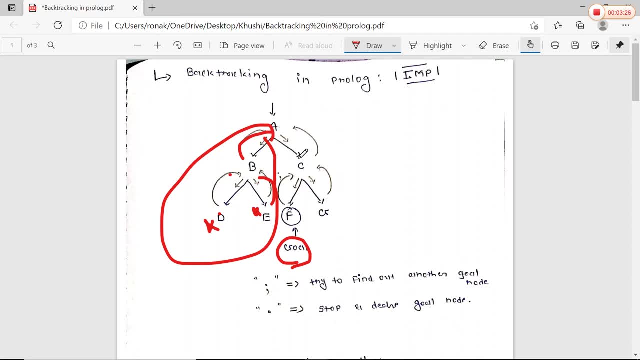 Now we have to move A2 to C. Now we have two options: Either left or right. So first of all we move to the left, Then move left As soon as we moved left, we got that our goal. node has been identified. 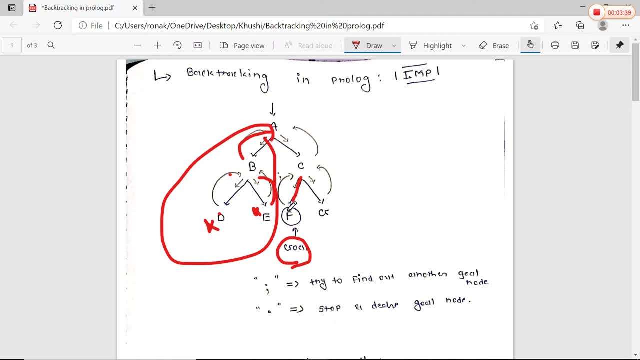 Now our goal node is identified. So we have to either stop here or then we have to check further whether there is a goal or not. So here I have identified one goal, but what did I do? again, I backtracked. 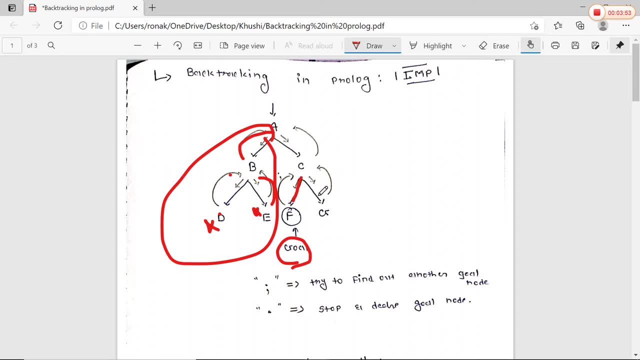 That means I went back again. I went to the right hand side of C to G. I checked it and it didn't come, so I backtracked and came back to A. that means I checked a whole tree, whole tree for the goal node and I have found one goal node as F. 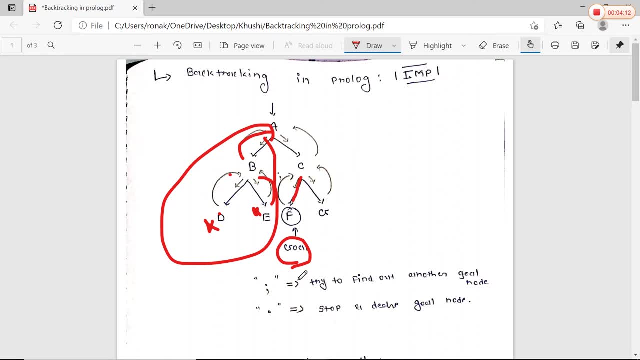 so if you implement this example and this sum in prologue, then you will have two options to identify your goal node. if you use semicolon instead of enter, that means OR. ok, semicolon is of OR and this is of AND. that means full stop here. that means AND. 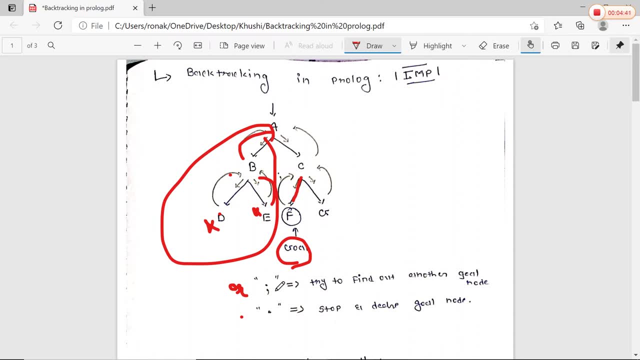 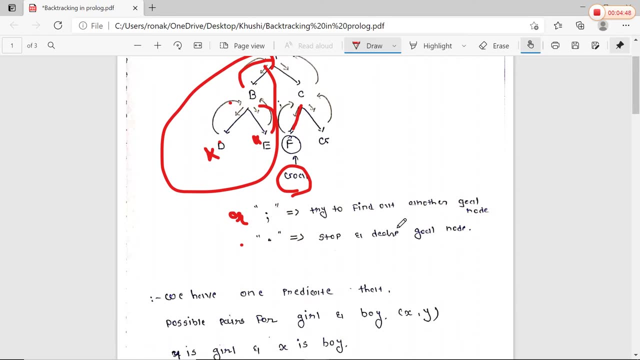 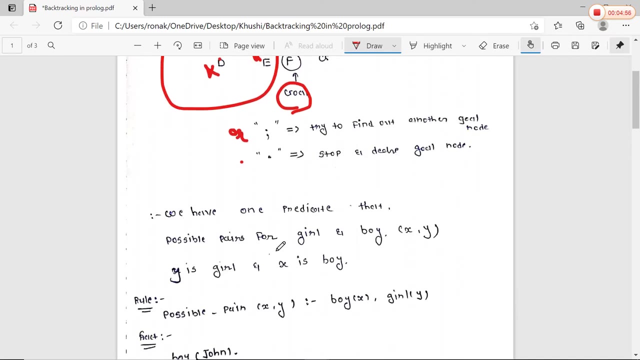 and if you have used semicolon, then OR another option is being identified or not to identify that. so semicolon is: try to find another goal node and dash. that means stop and reach our goal node. ok, we have one predicate that I have taken an example here. 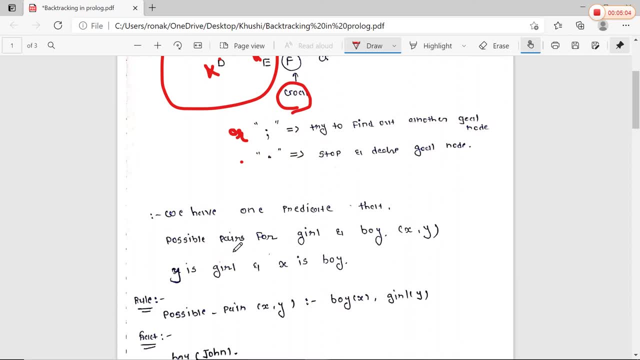 what is in the example? I have done in the example that we have to make pairs of boys and girls. so we have two girls and two boys. that means girls have X and Y is a girl and X is a boy. ok, what is his name? he has two boys. 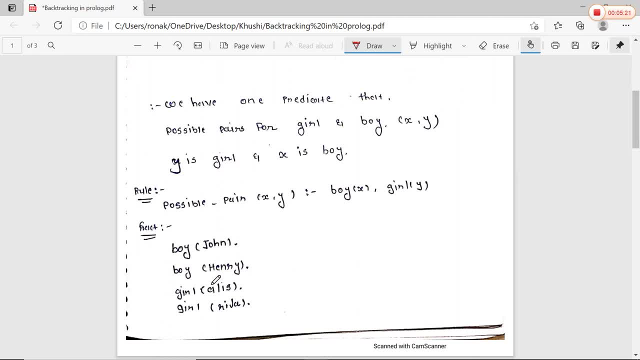 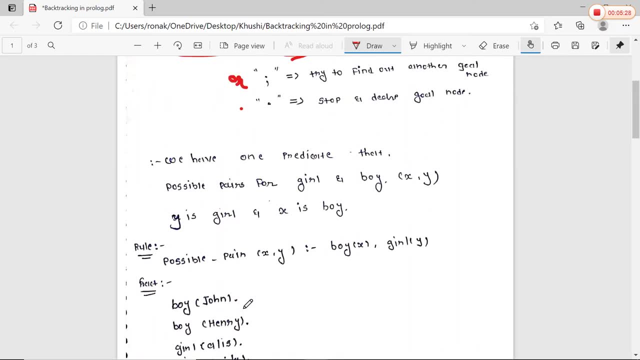 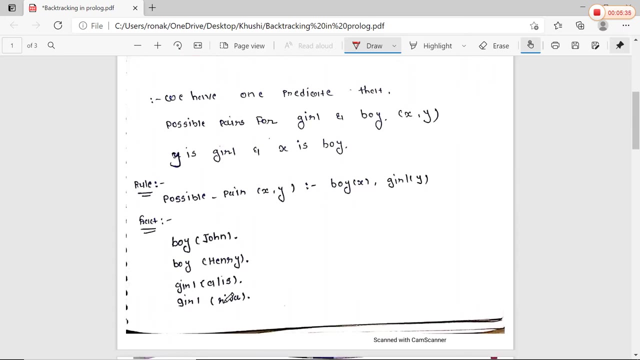 his name is John and Henry and there are two girls. his name is Alice and Riva. ok, so here I have. I have generate a possible pair, all boys and with all girls. ok, what I have to do is make John's pair with Alice and Riva. 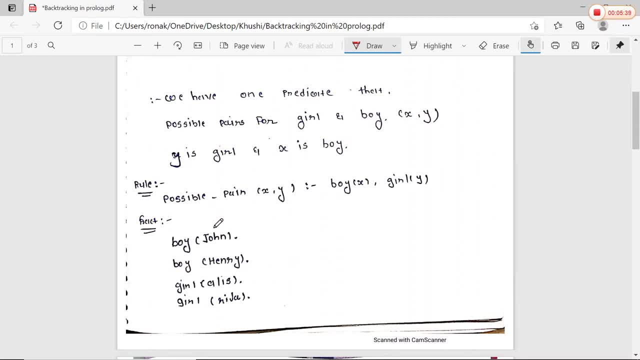 and make Henry's pair with Alice and Riva. that means don't make John's pair with Henry. boy and girl. boy and girl. I want to pair with another means the opposite of him. I want to make his pair with her, not boy boy's pair, I want to make a pair of boy and girl. 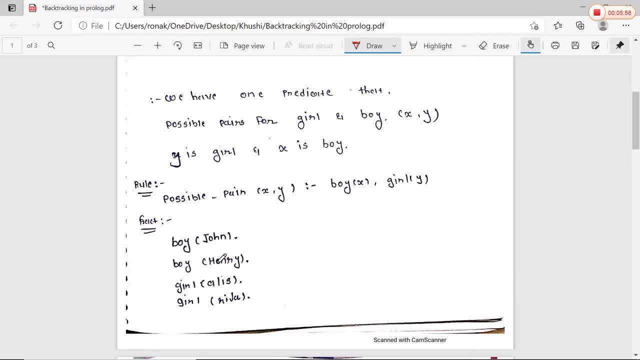 so here, what is the possibility? there can be a pair with John's Alice, there can be a pair with John's Riva, either with Henry's Alice or there can be with Henry's Riva. if it is with John's Alice, then it can't be with Henry's Alice. 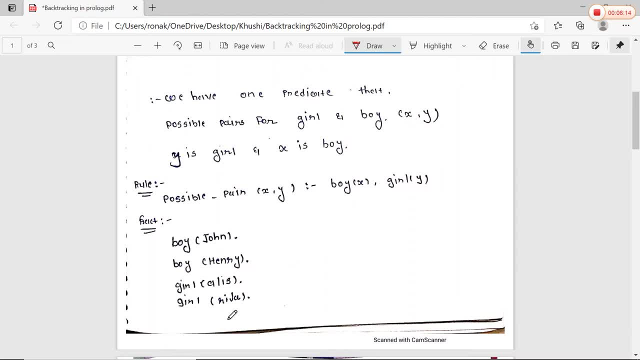 and if it is with John's Riva, then it can't be with Henry's Riva. ok, So our total possibility is 4 pairs, with John's Alice, John's Riva, Henry's Alice and Henry's Riva. So my predicate possible pair is equal to boys x, girl y. 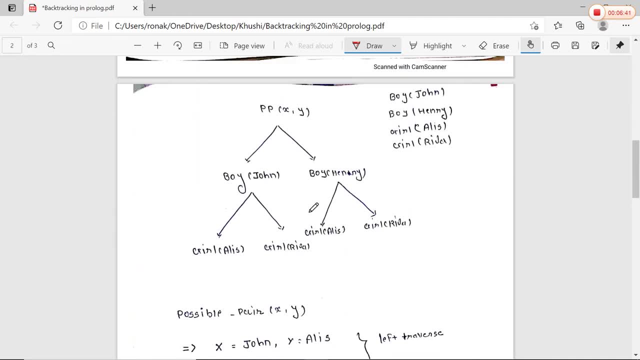 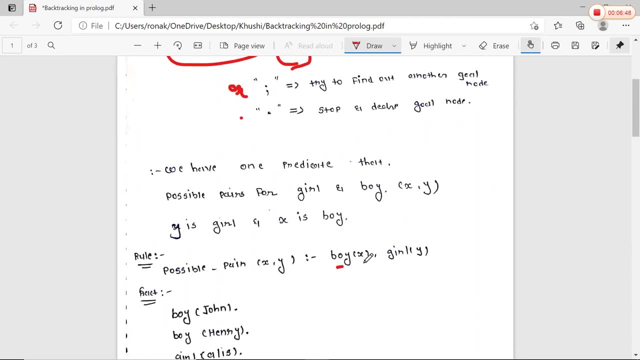 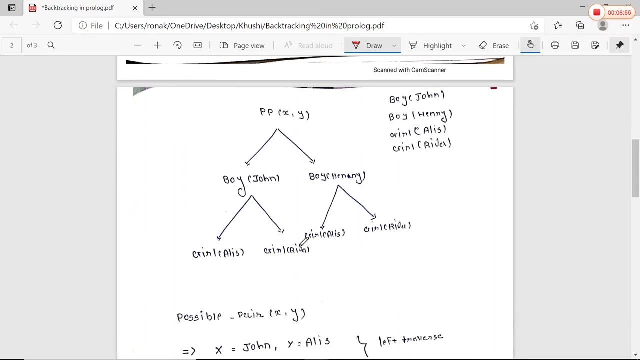 Here I have generated a graph. So my predicate possible pair is x, girl y. This one is my root node. After that, which predicate is being used here? First of all, boys. So which node have I visited here? Boy John and boy Henry. 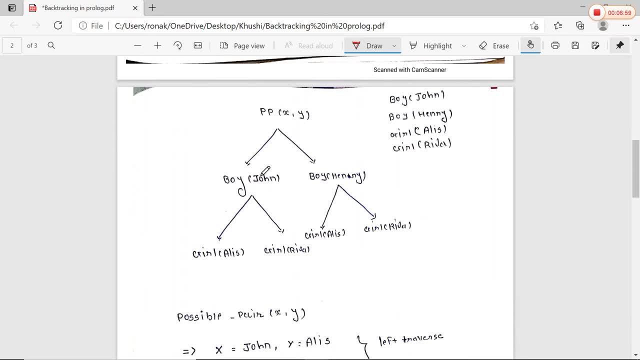 Here boy John, Henry, Alice and Riva. After that I have to make John's pair with Alice and Riva And Henry's pair with Alice and Riva. So I made John's pair with Alice and Riva And Henry's pair with Riva. 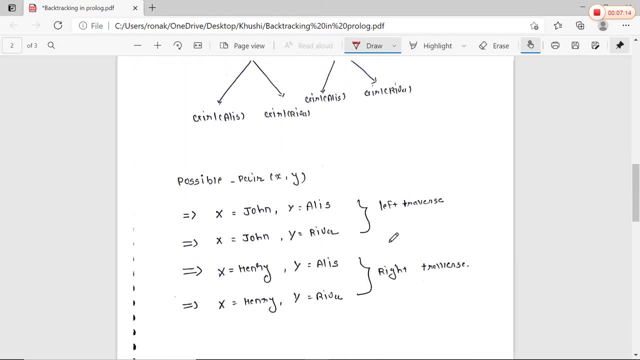 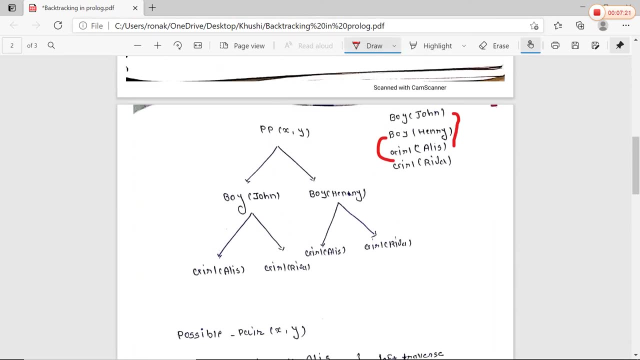 So I made John's pair with Alice and Riva. Now what is my possible? So if I do left travel without backtracking, I take one here Now. here, first of all, what I do. I go above boy John with possible pair. 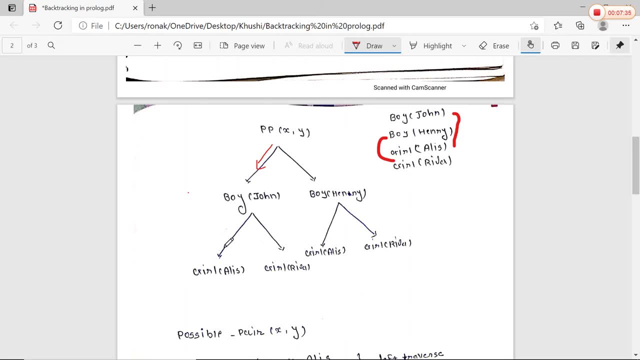 I get no option from boy John. Either I make boy John's pair with Alice or with Riva. Either I make boy John's pair with Alice or with Riva. Either I make boy John's pair with Alice or with Riva. If I make boy John's pair with Alice, where will I go after backtracking? 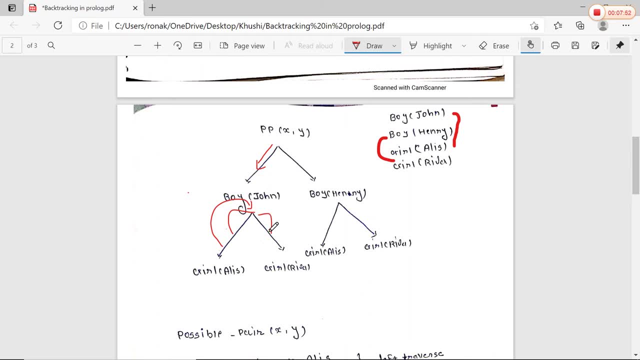 To John, And where will I go after? To Riva. What will I do after going to Riva? I will backtrack him And where will I go To John? And from there? what Backtrack Now? what is the next option? 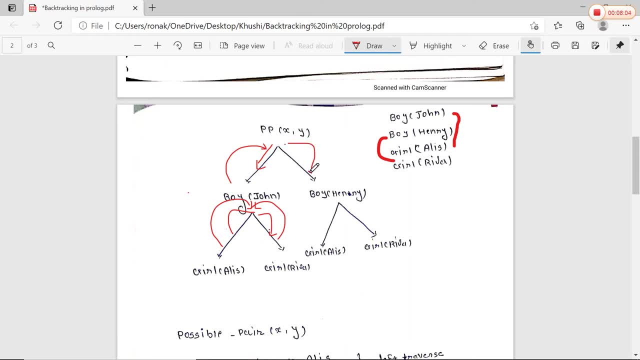 I have to make Henry's pair. I have to make Henry's pair With whom? First of all, I will make it with Alice. Okay, I will make it with Alice. After that, I will backtrack. After backtracking, what will I do? 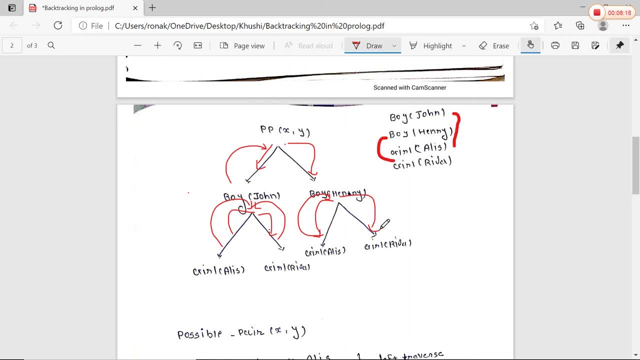 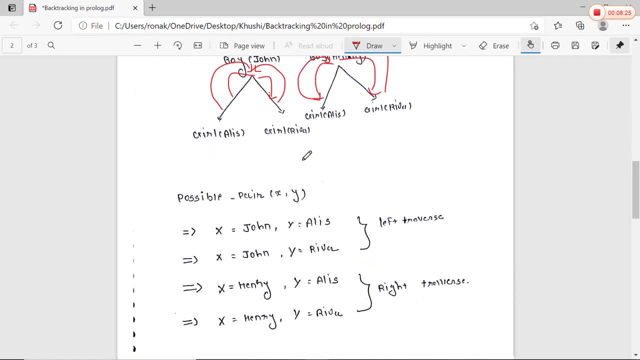 I will go back to Henry and make it with Riva. After backtracking Riva, I will make it here, And from here I will backtrack. Now, what did I get? I got my pair. What kind of pair did I get? 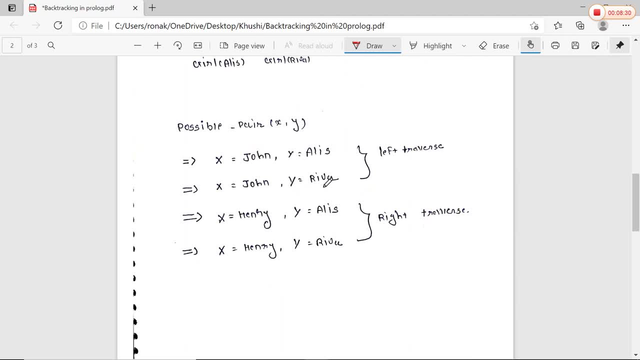 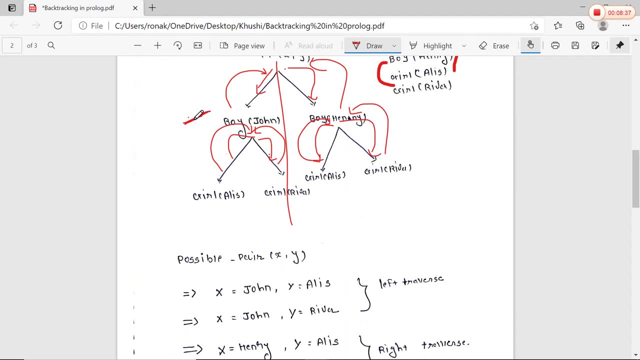 What is the possible pair? John with Alice, John with Riva- Okay, This one is the left travel Left travel. That means this, This part of left travel, Left travel, Okay. And another one is the Henry with Alice and Henry with Riva. 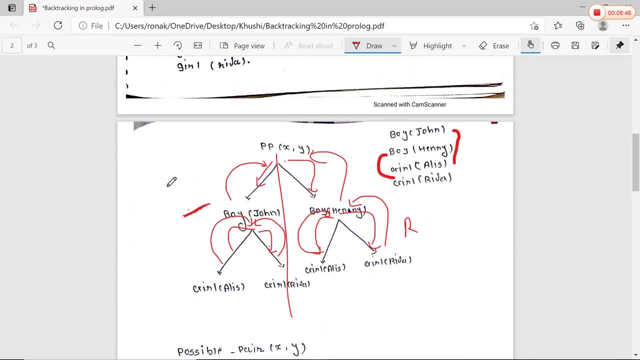 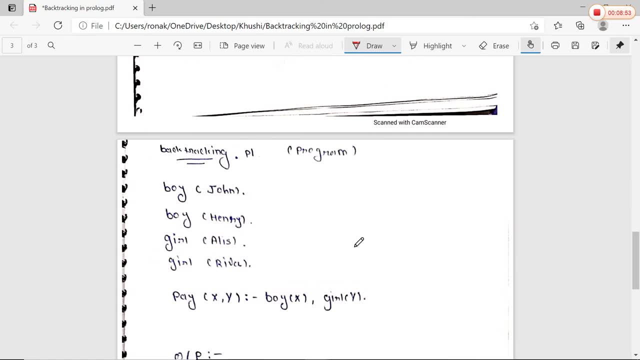 So this one is the right- travel Okay. And this one is the left- travel Okay. So this one is the right and left, both are travel. Here I have summed up this example, that how you have to run in prologue. 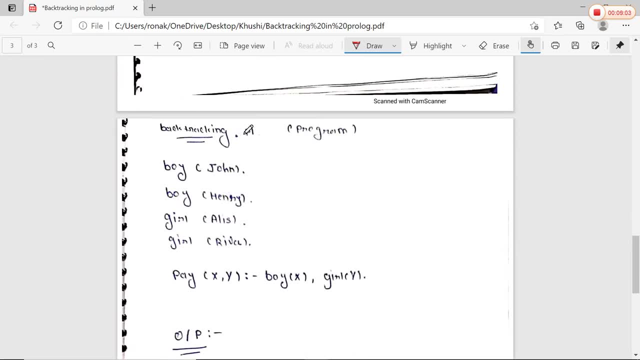 So, first of all, what you have to do is make our knowledge base- What is in knowledge base- Backtracking. I have given the file of PL here. That means the file of prologue. You can give the name of any file. 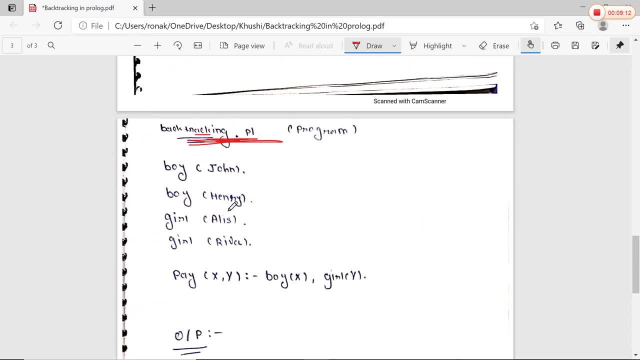 I have given backtracking here. You can give any file. What did I do in my knowledge base? In my knowledge base I added that John is from boy, Henry is boy, Alice is girl, Riva is girl And my predicate. that means: what is my fact? 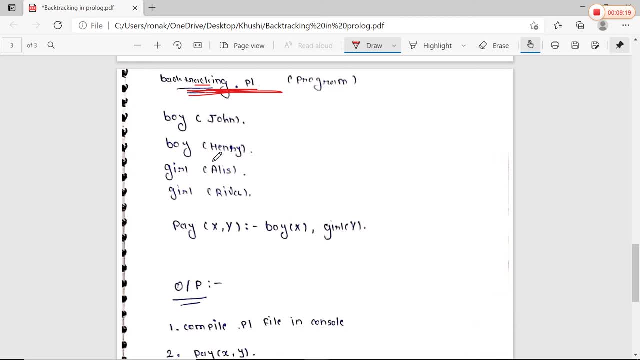 Pay x, y Means pair x, y implies boy x, girl y. Okay, Now what I have to do: First of all compile, Then this function. So here I have to compile. So here I have to compile. 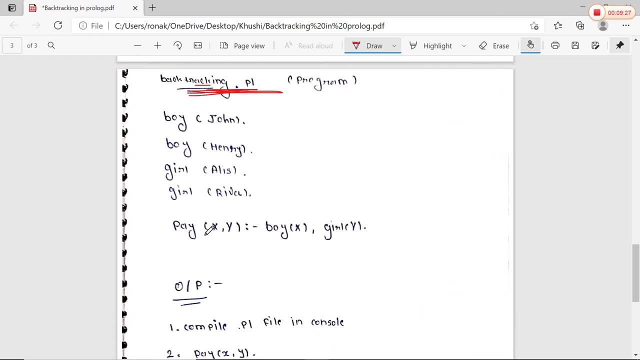 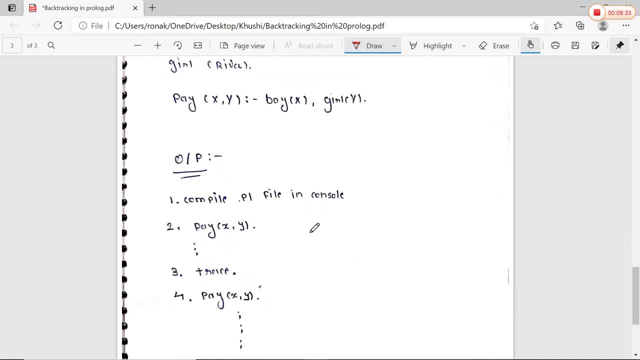 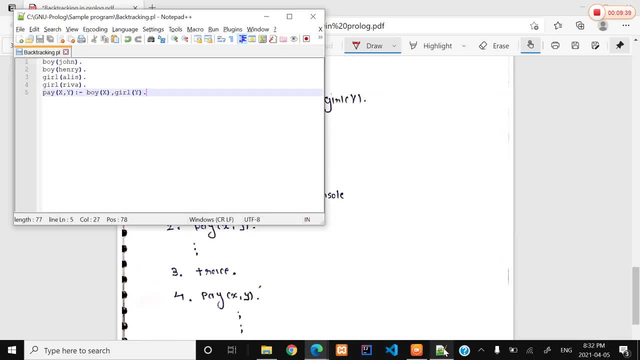 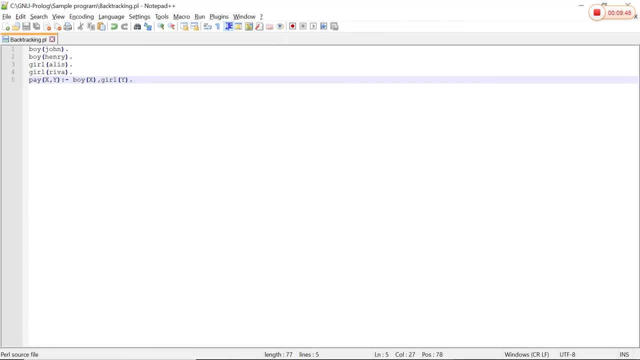 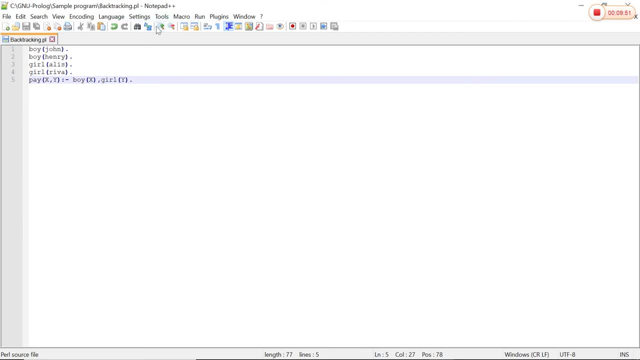 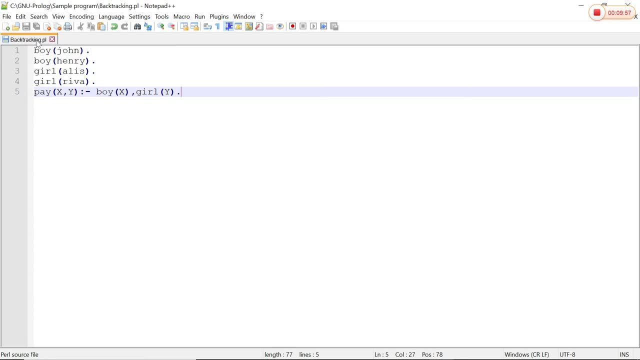 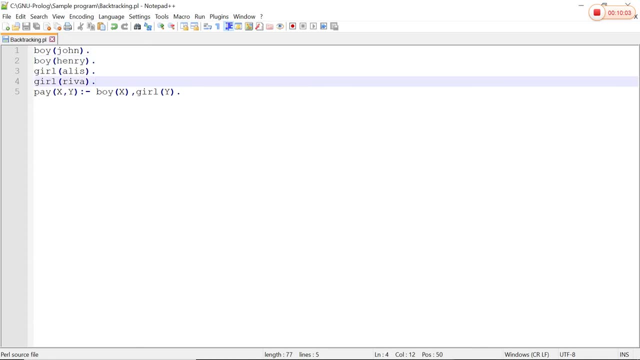 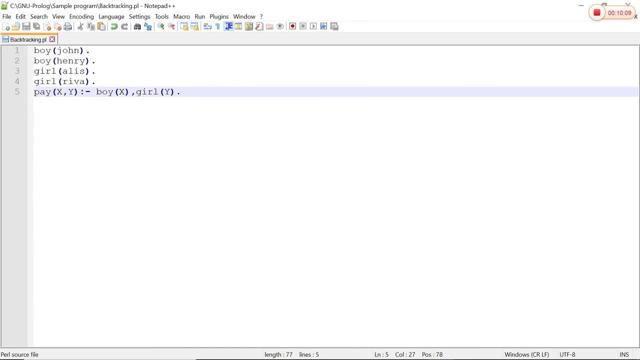 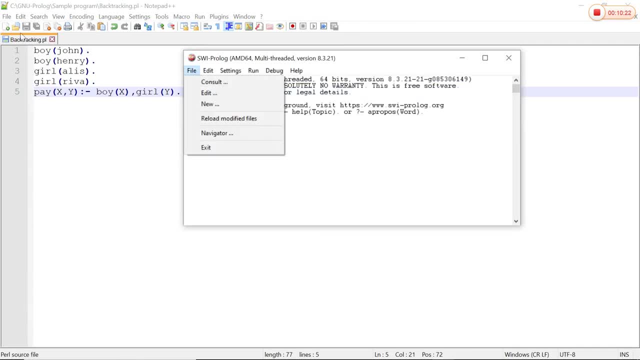 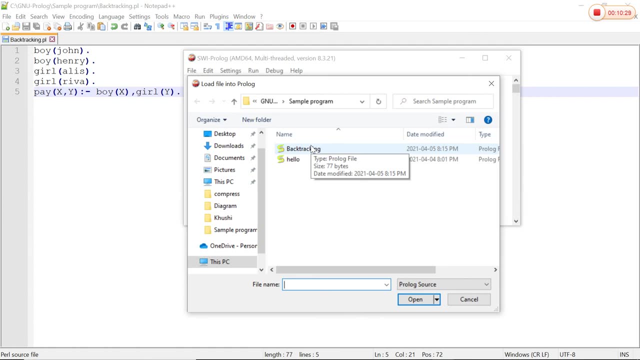 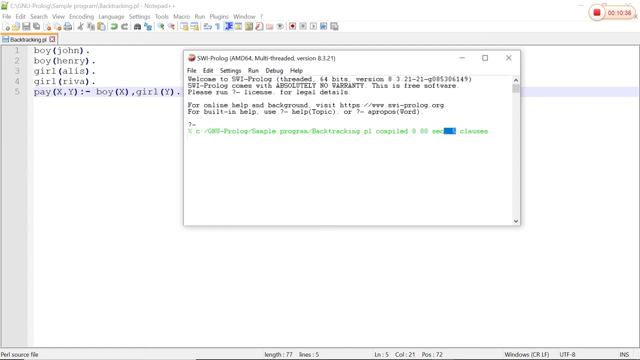 open swf prologue. after that I have to compile this file. open console where your backtracking file is. you have to open it. successfully compiled file is closed because our line is of 5, so its 5 is closed now. what you have to do now? you have to check this function. 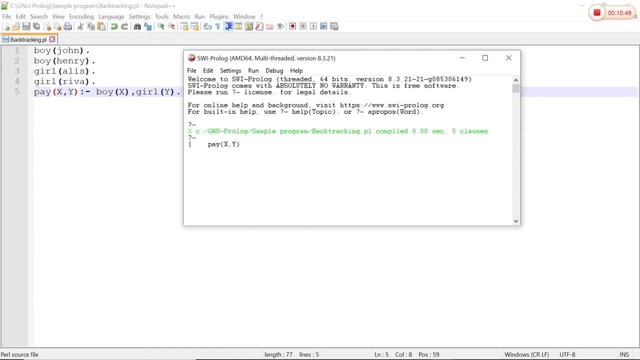 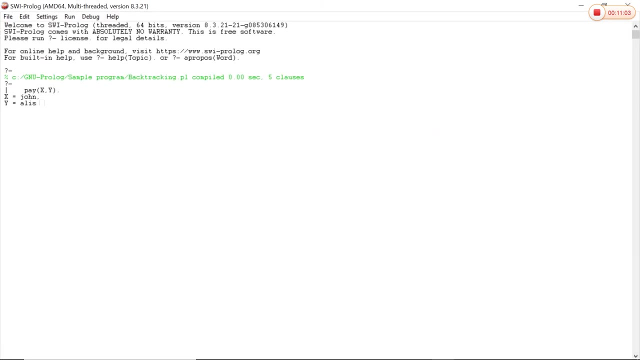 that means pay xy and dot for the ending of the statement. so what he did? he gave me the value of x and y pair. if I press enter. if I press enter, then what will come? he will understand it as end. so what did he say? he understood it as end. 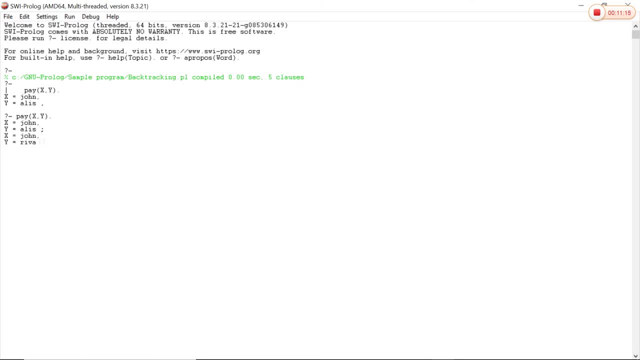 but if I don't press enter, I am giving semicolon. so what did he do with John's Alice, John's Riva, with Henry's Alice and Henry's Riva? what did he do to me? he gave me the pair. now what I have to do. 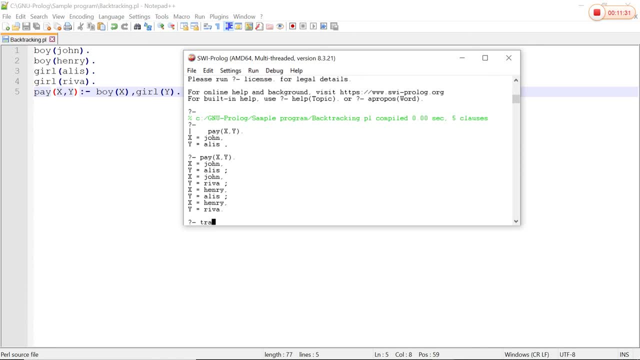 I have to trace. how does he backtrack? that means, how does he trace his one by default function is trace dot to end. so what did I do? with whom I have to trace? I have to trace this function. so see here, first of all, what did he do? 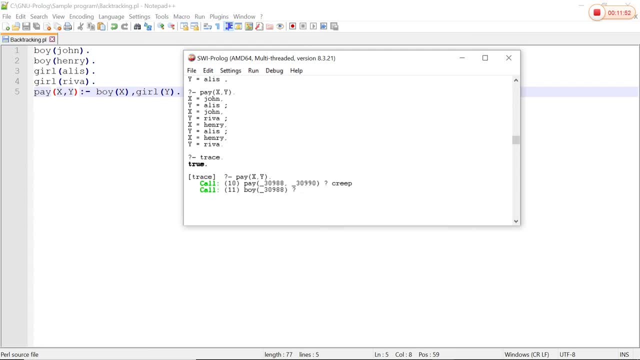 he started with our first. what came in that boy came one value of John and Henry. ok, from that first value of John he started. that means 98080 and 990. from there he started with John, so he started with John. if I press enter, then what will come? 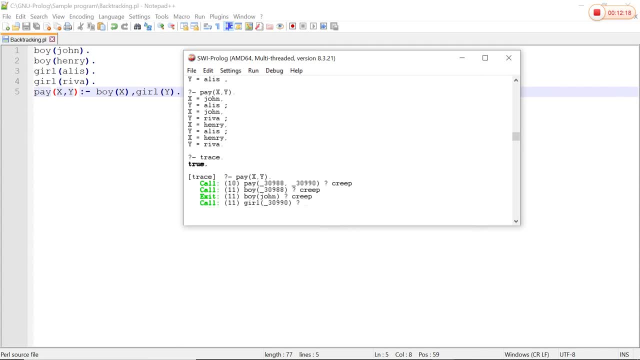 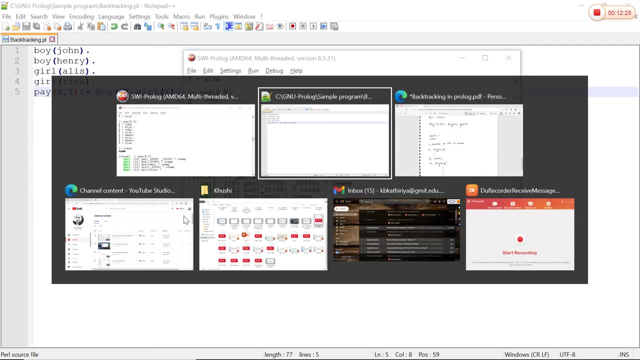 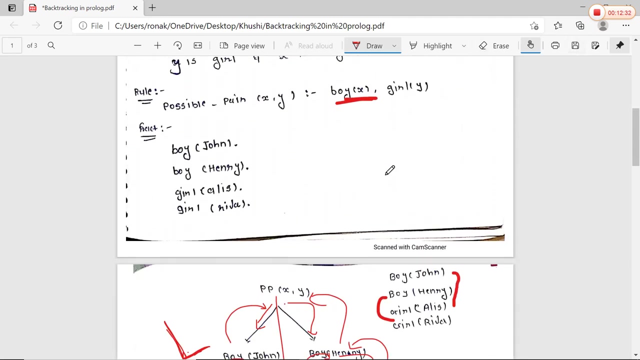 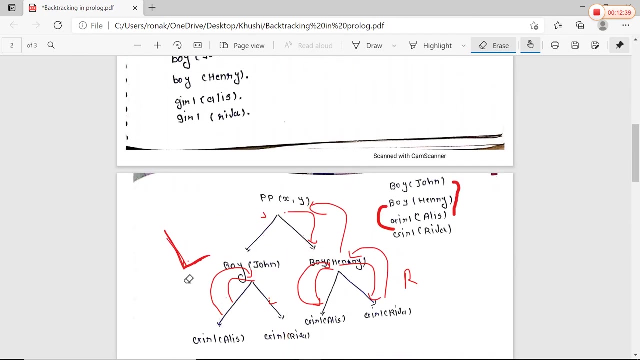 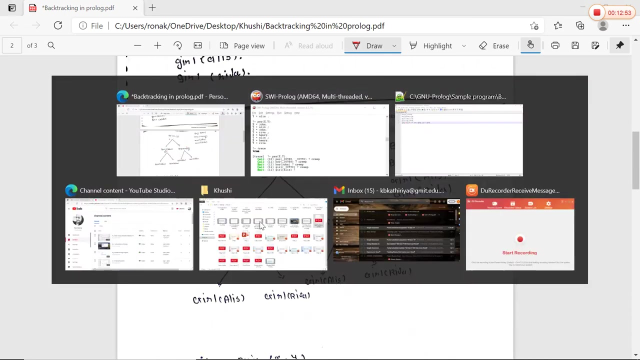 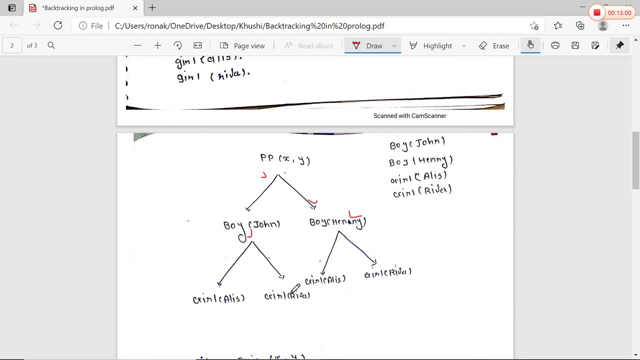 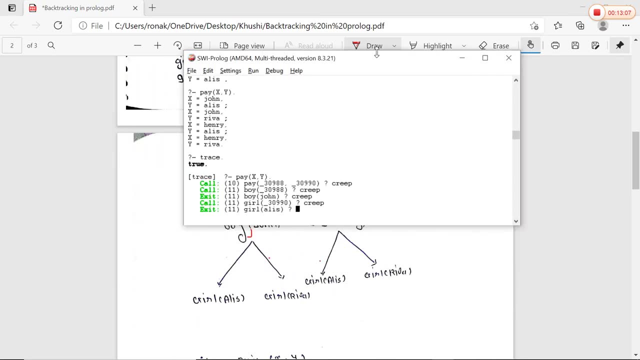 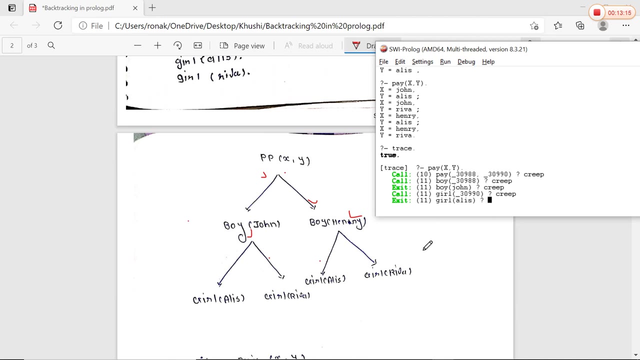